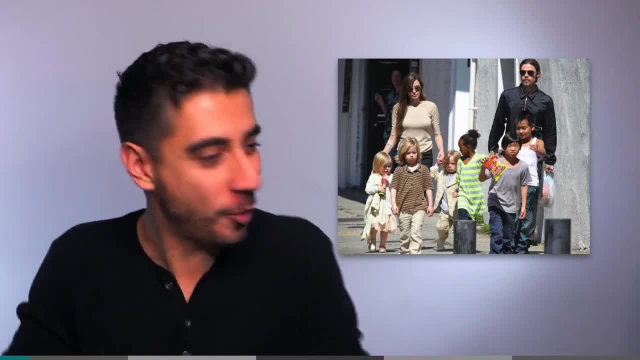 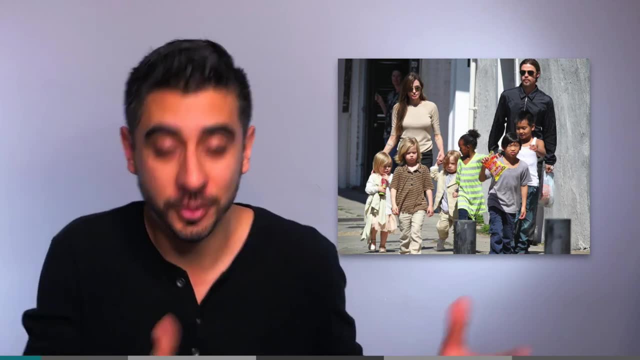 old enough to go to school. Look at all these beautiful babies from all over the place. First you have to pick the right kid, the one that's old enough to go to school, and then dress them or style them or prepare them for school. That's what. 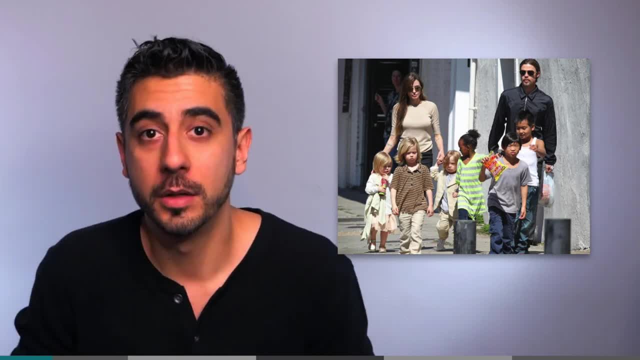 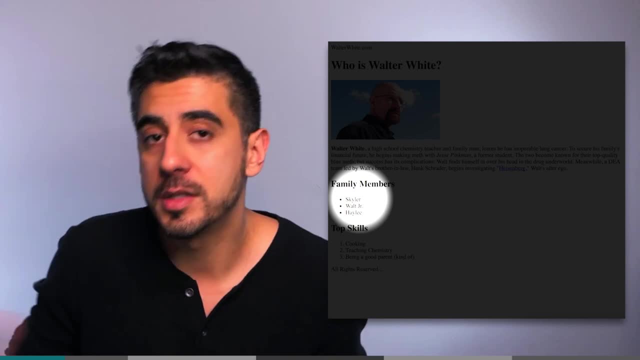 selectors are: Choose which kid you want to prepare for school or, since you're not Brangelino, choose which element you want to style. It's the same concept and it all starts with the selector. There are different kinds of selectors In our 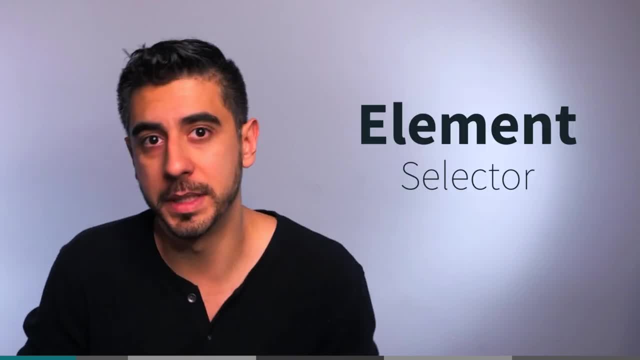 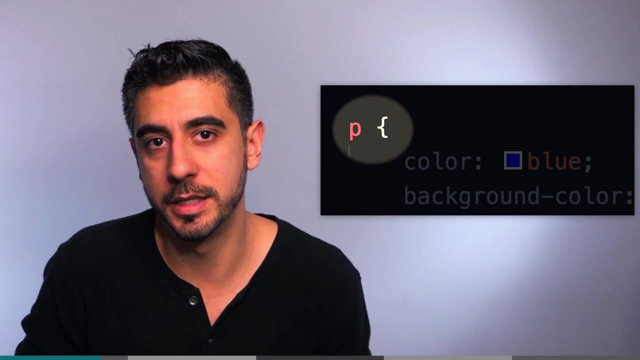 example, in the last video we use what's called an element selector, because it targets your style based on the element type itself. That's the most basic selector. there is the element type, like a p, cool, cool. the problem with element selectors is that you might not want. 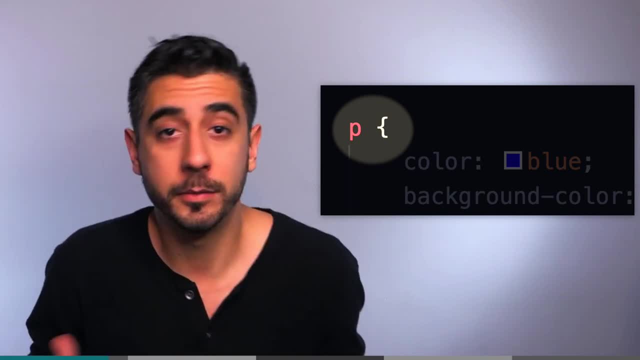 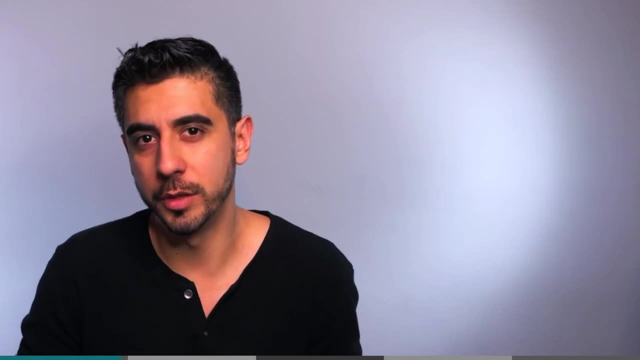 to turn all your paragraphs blue? what if you had three paragraphs and you only want one of them to be blue? the element type is an identifier, but in this case it's too general. i want to show you a real world example. look at this on adam's website. see these two sections. one of them has a. 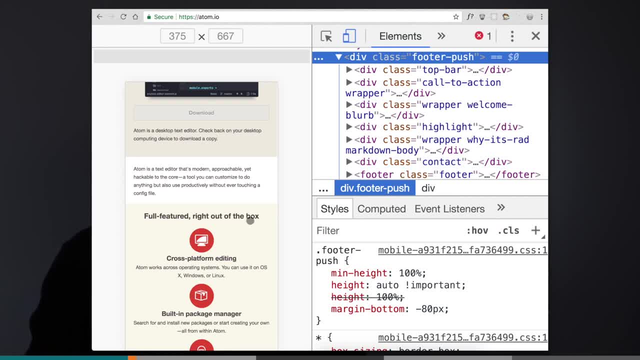 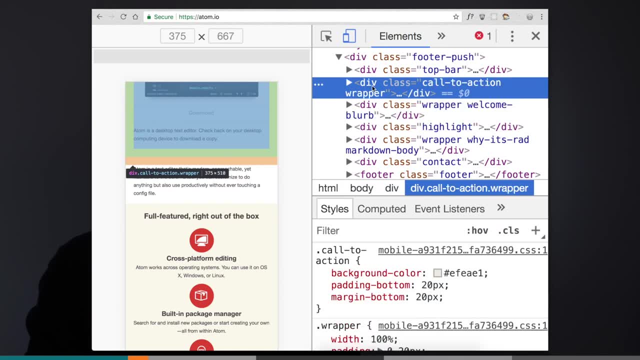 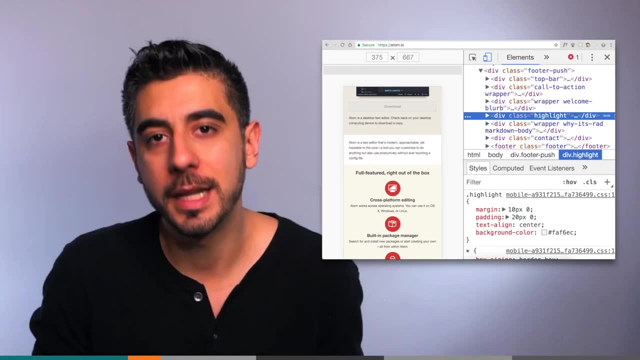 white background, the other one is beige. if you inspect it, you'll see they're using divs for both of them. so clearly the guys that made this couldn't have said, oh, select all the divs and change the background to white or beige. they needed to be more specific. you can select elements. 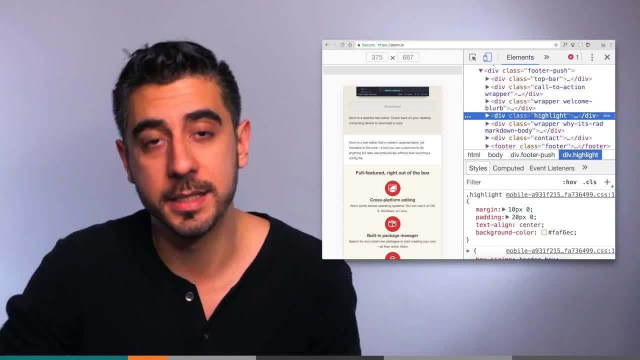 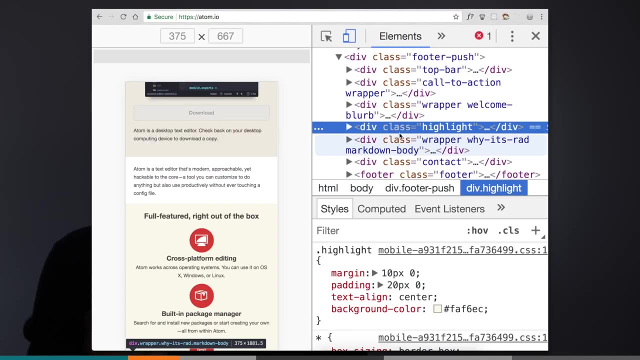 based on other kinds of identifiers, classes and ids class is the most common and useful one. in fact, that's exactly what adam is using. take another look. they have a wrapper class on one and a highlight on another one. if you click on the div with highlight class on it, you'll see that the 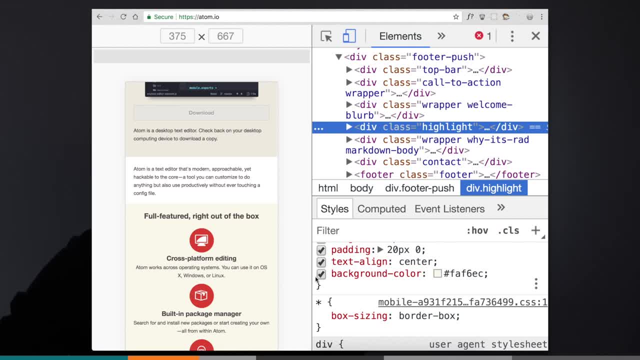 class has a different class, and you can see that the class has a different class, and you can see that the class has a different class and you can see that the class actually has a style that includes background beige. it's right there. so let's do one ourselves. let's say: you have 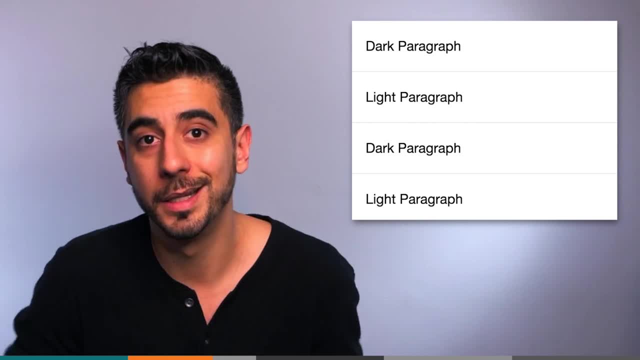 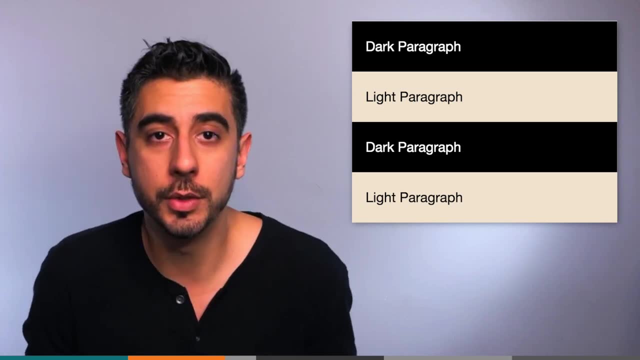 four paragraphs and you want to alternate between dark and light. so dark light, dark light. in other words, you want to reuse a style for multiple elements. in this case, you can use a class selector. the way you write these in css is you write the name of your class. 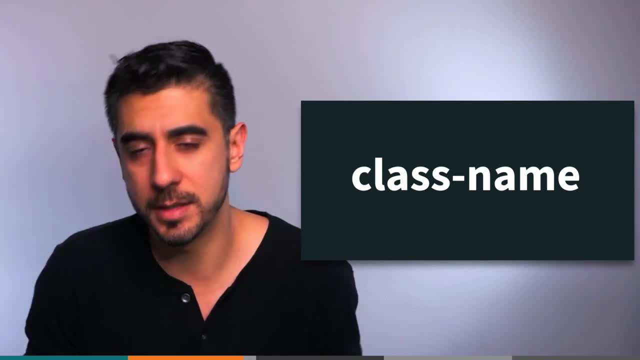 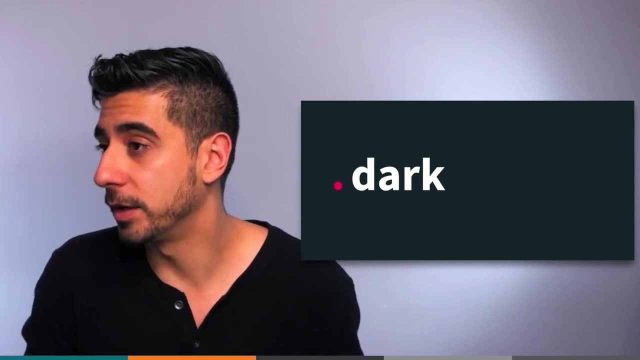 this could be whatever you want, just you can have spaces and some special characters say dark, and you put a dot in front of it. why a dot? well, i don't know what to tell you, it's just syntax and you just have to remember it. this tells the browser: hey, this is a class selector. and then 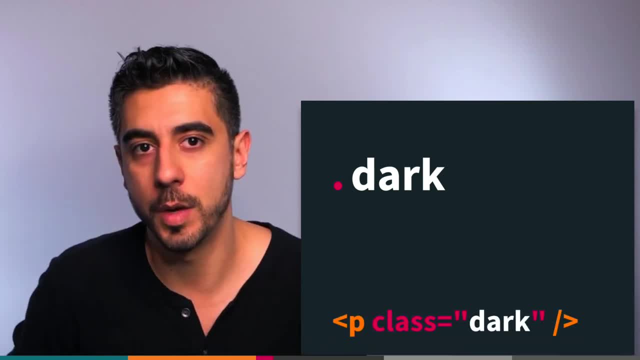 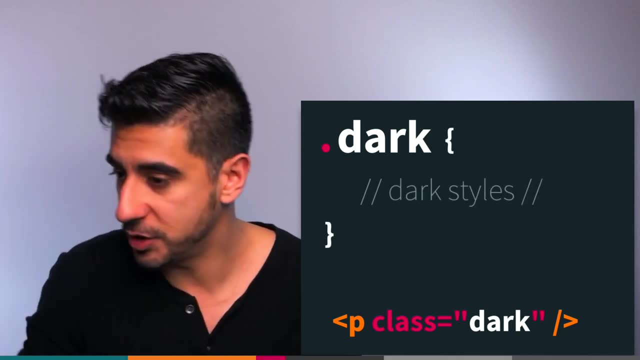 of course, you have to add that class to your html element as well. this means, hey, select all the elements that have a class attribute and the value is dark. so let's try it ourselves. uh, so i have four paragraphs here. i've added dark light and i've added dark light and i've added dark light and. 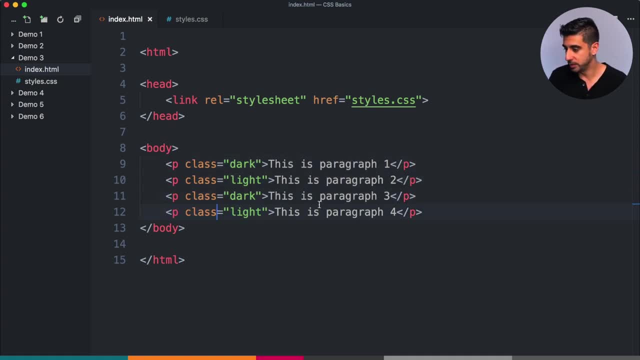 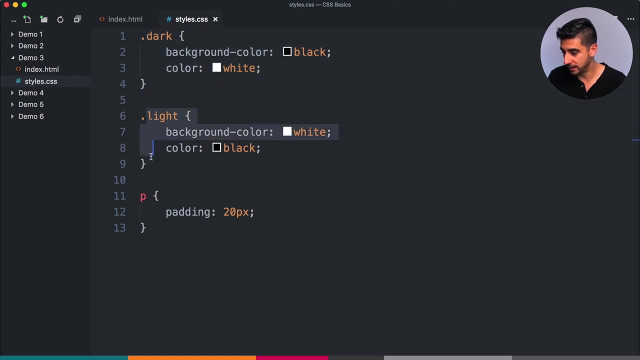 dark light, dark light classes to them. so you can do the exact same thing that i have, same thing as the last video. i have a stylescss file that i'm linking to and, if we take a look at that guy, i have two classes: i have dark class and i have a light class. so the dark class has 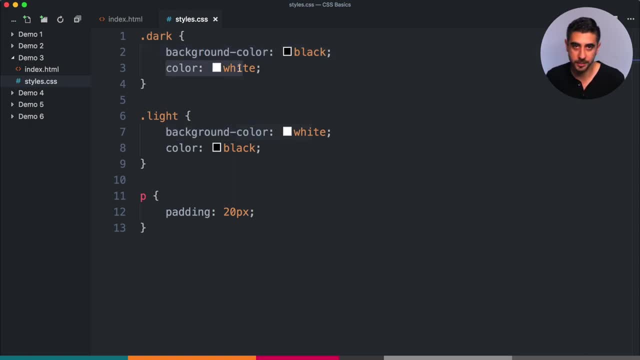 background color black and color which is text color, you should notice by now- white, and the light selector, or the styles for my light class, are the exact opposite: background color white and text color black. i also added a padding of 20 pixels to all p tags. uh, just so you can see it. a. 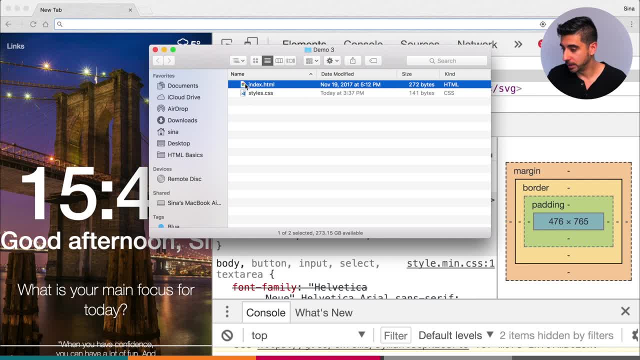 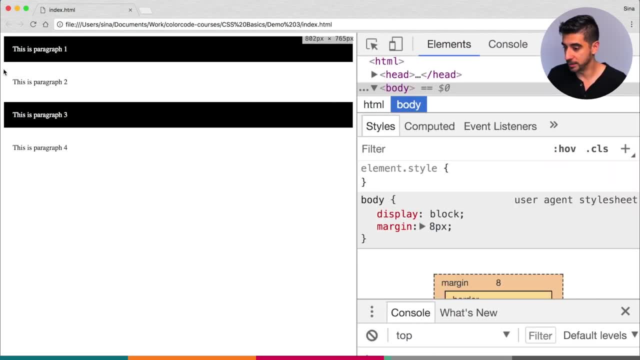 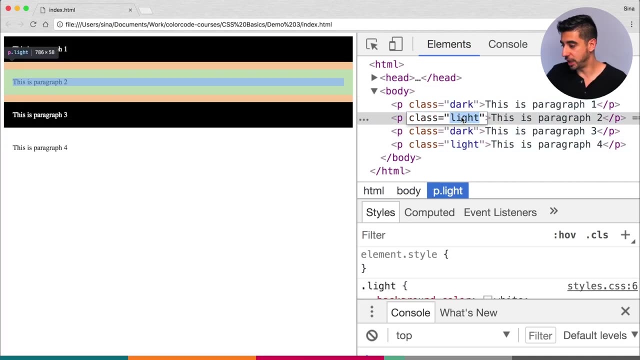 little bit easier. so i'm going to go here. i'm gonna open this file and look at this. we're alternating between these two styles, right, and what's so awesome about this is that you are reusing dark and light as much as you want. you can basically change any of them. you can change. 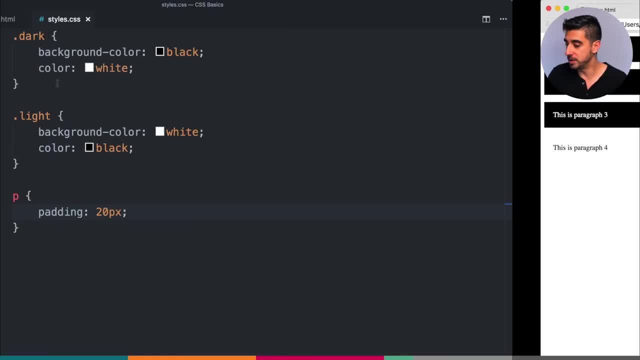 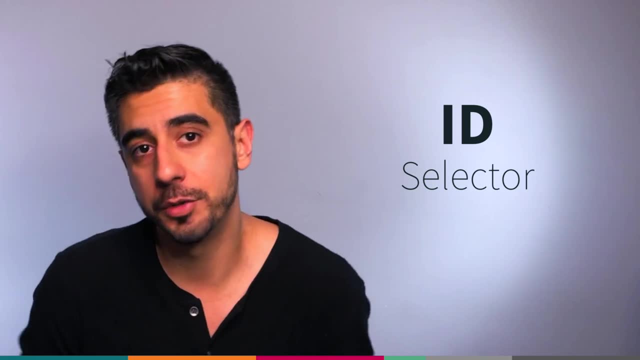 the second one to dark, and that's now going to be dark right. reusability, my friends. i'm also going to cover id selectors too, just for the sake of it, although we don't use them that much. id attributes are specific to one element only, if you have a style that you want to apply to only one element. 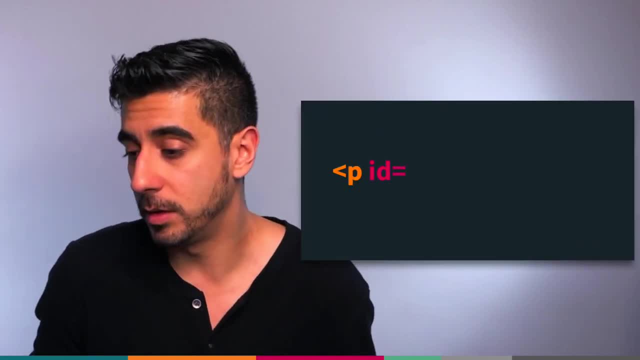 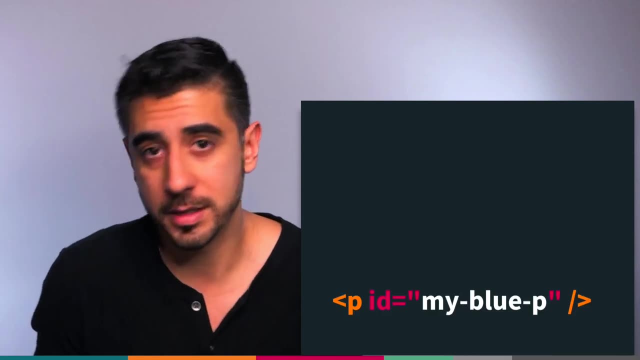 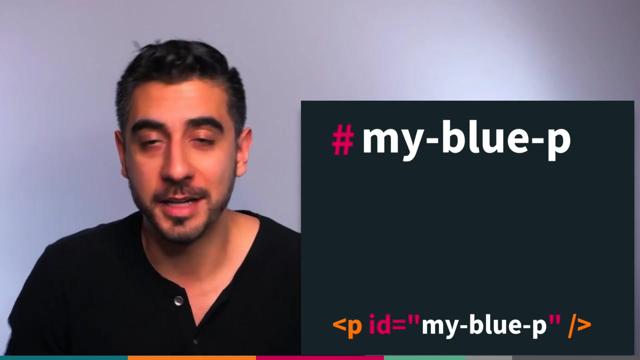 for some reason, you can add an id to that element, for example my blue paragraph, then use an id selector in css to style it. id selectors are just like class selectors, except you put a hash in front of the name instead of the dot. i don't know how to explain it, it's just syntax, so that becomes.